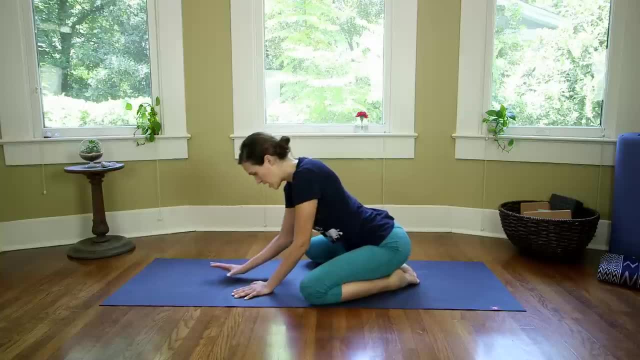 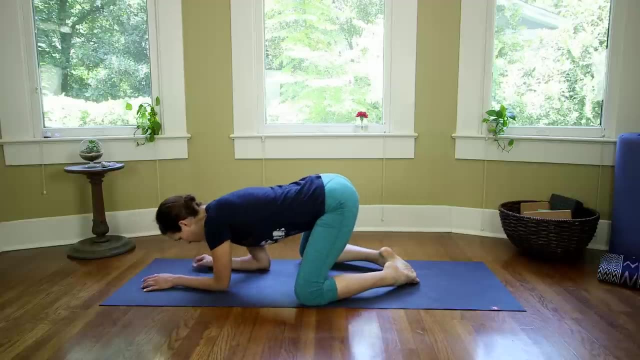 pose. so get on down Knees as wide as you can. Side is your mat, Two big toes touching Now. if this is like not a comfortable posture for you, then you can keep the hips lifted and in time, baby, we'll get them down. 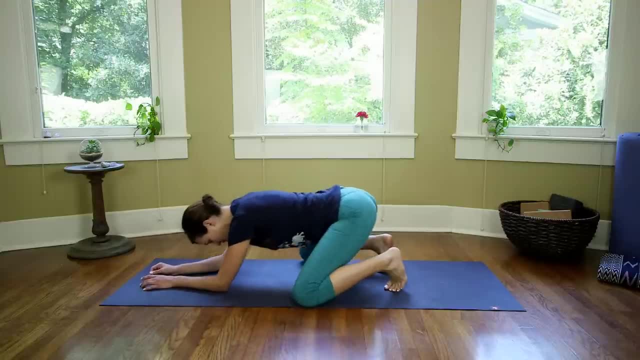 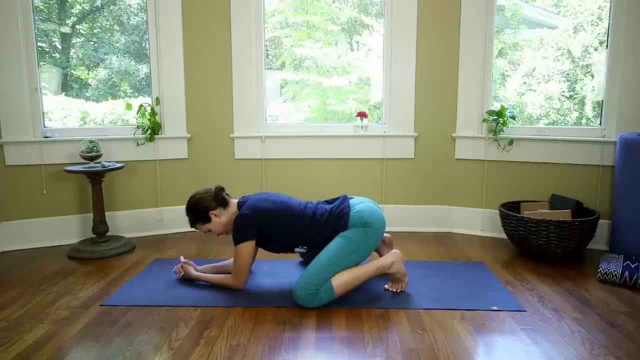 there. So just be where you are at today. If you need to curl the toes under and stretch the feet and just kind of rest on the elbows, this is an option. So just know that your extended child's pose may not look like the magazine today, but it will evolve and change, so you just 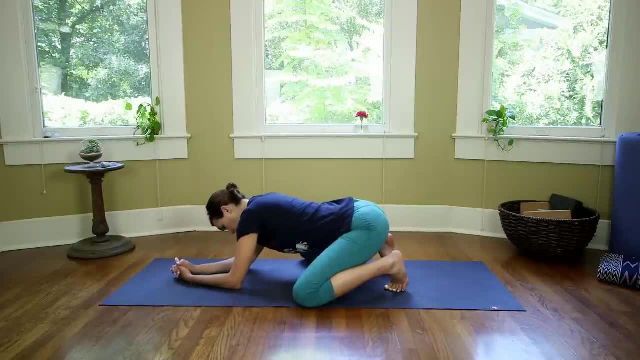 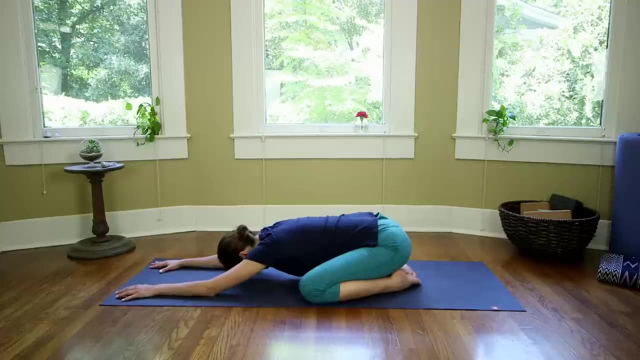 kind of have to get into it, and so that's where we're starting. We're starting today just kind of nice and easy in an extended child's pose. If the forehead can come to the mat, you might experiment with that, melting your heart down. 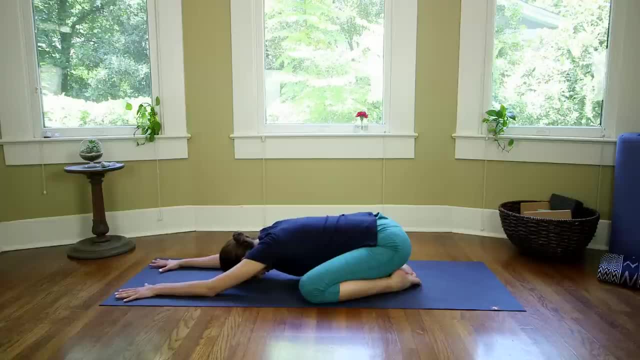 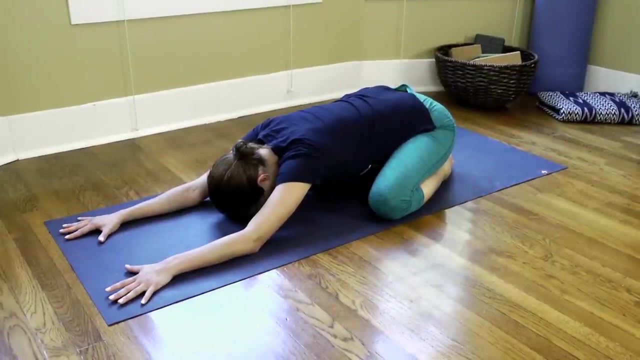 And just take a second to close your eyes and draw your attention to your breath. A little invitation to notice the breath is super important here. as we begin today And talk about vinyasa, or introduction to, you know, flow style yoga and just the synchronicity that comes when 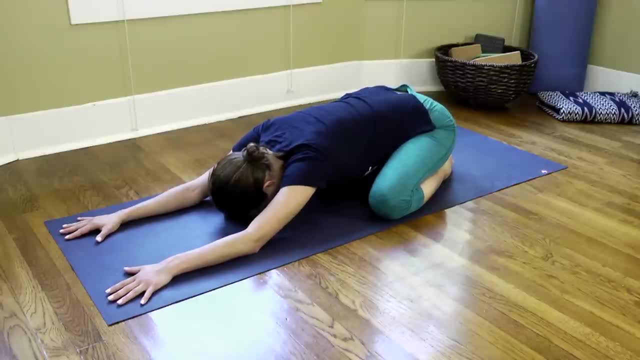 you start to really, you know, play with your breath and move with your breath and let your movement be fueled by the breath is so rewarding, especially in a physical practice. It's like totally the manifestation of joy, And if you don't know what I'm talking about yet, you soon will. 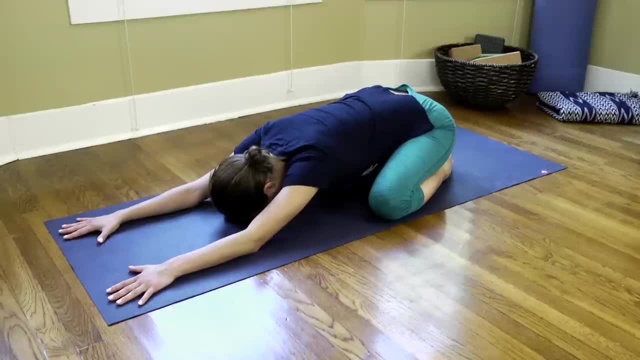 You do, and you know I'm not crazy. Notice your breath, Take it nice and slow. We're going to move in a circle here, so the goal today is to not do it perfect, but to just enjoy the ride. stick with the. 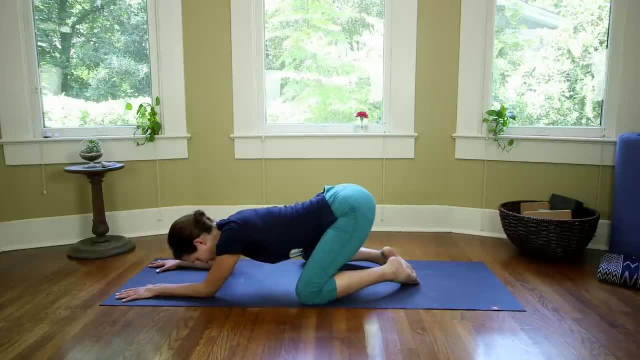 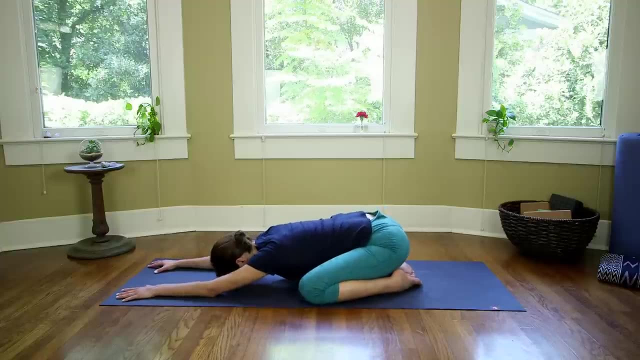 practice. so we're going to start by inhaling coming forward and exhaling around and back. See if you can move with your breath: Inhaling coming forward, Inhaling coming back, Inhaling coming forward and exhaling around and back through. 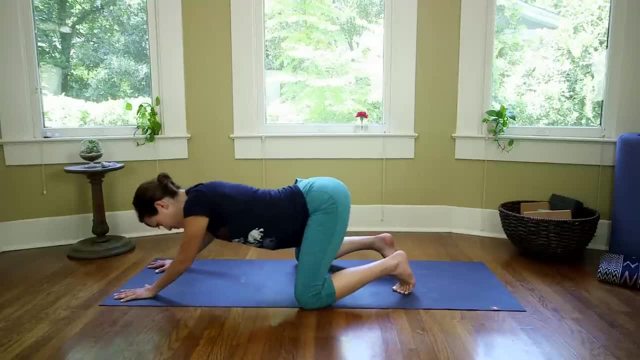 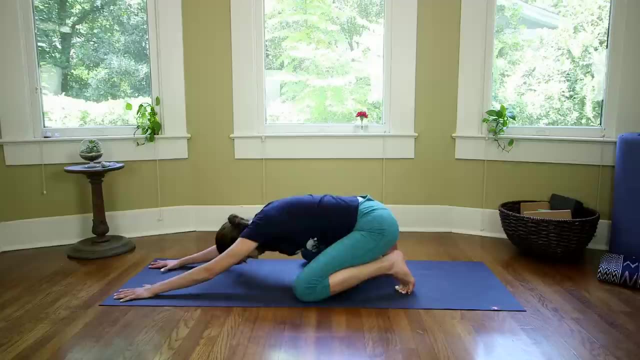 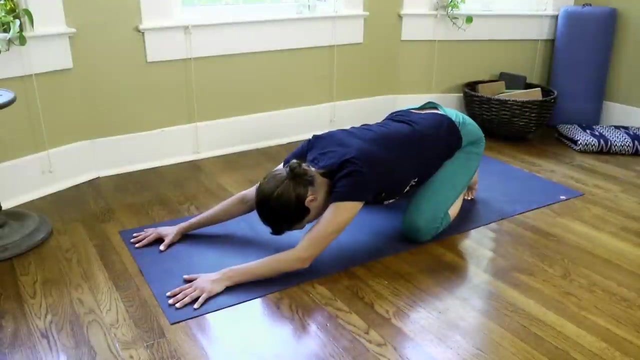 that extended child's pose. Keep it going, Inhale, come forward, Moving in a big circle, exhale around and back and then reverse your circle again, inhaling as you come forward. Exhale through extended child's pose. 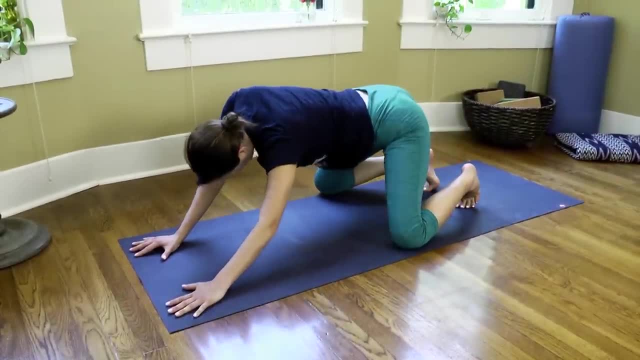 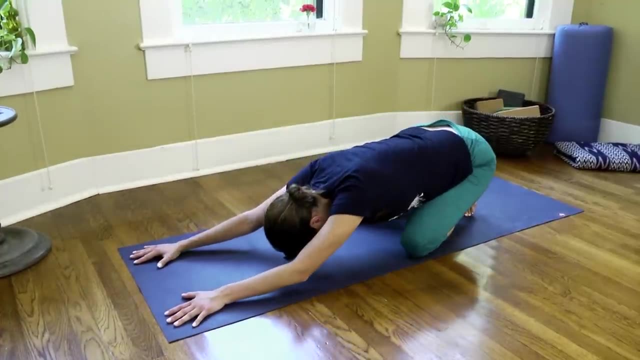 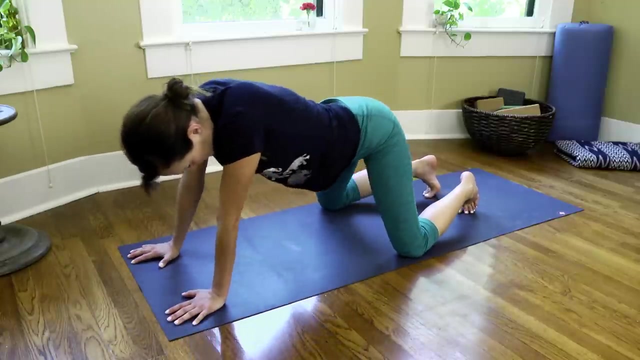 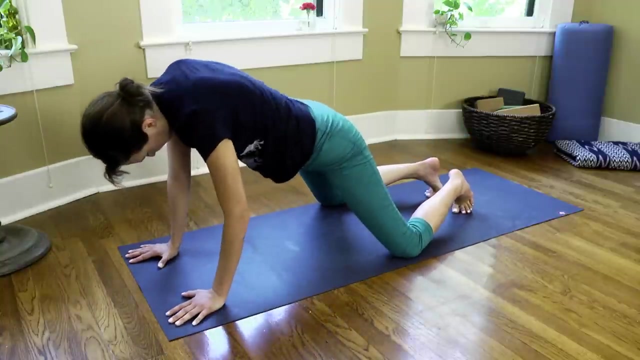 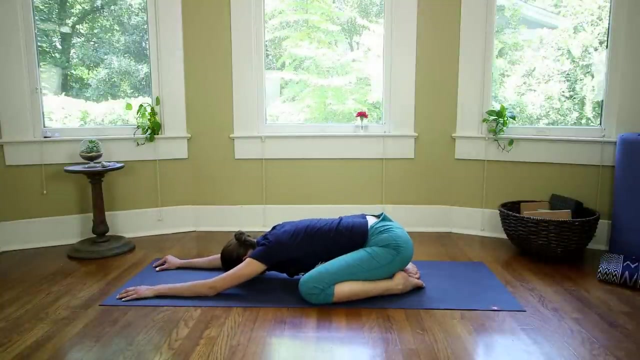 Now we want to take long, deep, smooth breaths- so rushing your movement isn't really great for that- and slow it down so you can kind of focus and begin to control the breath and the movement. Let's do one more And back to extended child's pose, or your version of extended 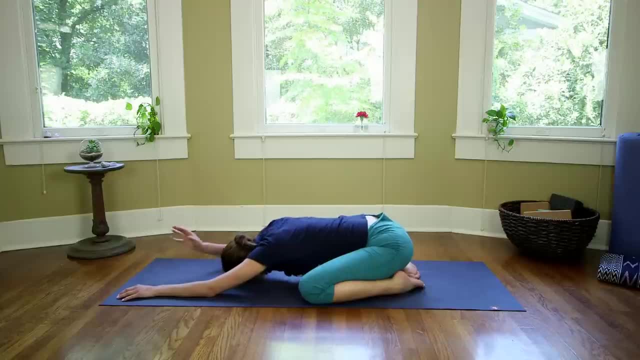 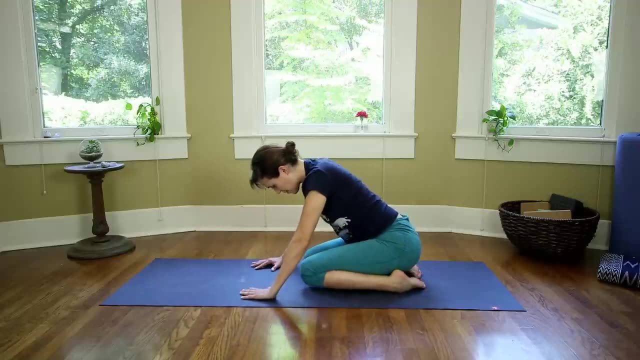 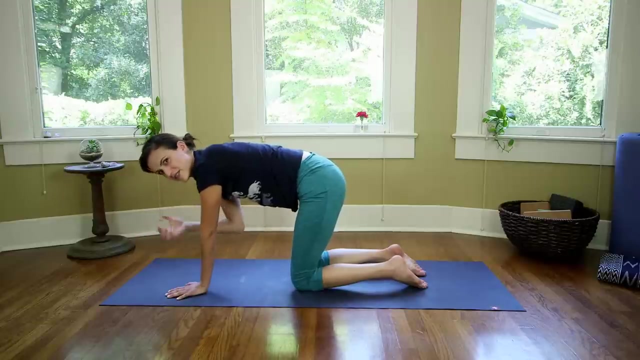 child's pose, Awesome. Then we'll gently draw the palms underneath each other, Keep the shoulders and press up. Walk the knees in line with the hips and press up. Come to all fours table top position. Just a little side body stretch, since we're going to kind of hop. 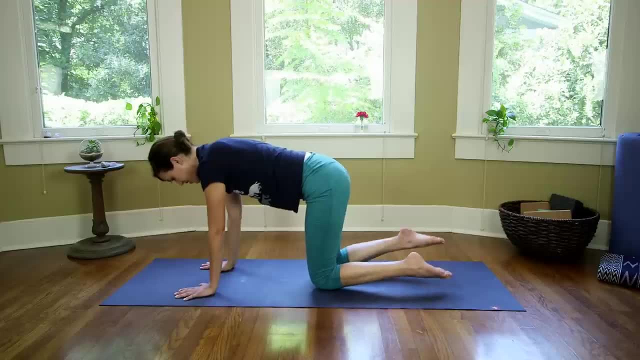 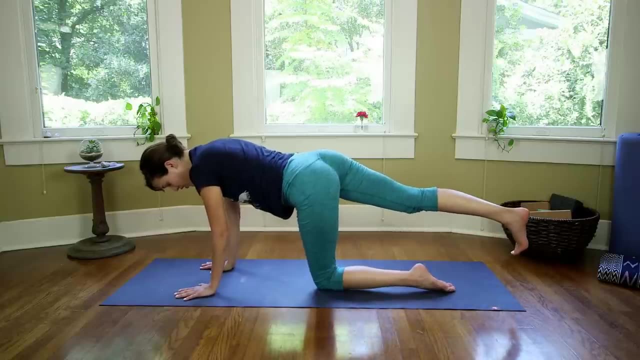 into a flow today kind of quickly. I'm going to press into the tops of my feet- but you're going to be okay- And I'm going to extend my right leg out. Take a deep breath in On an exhale. draw your right toes over towards the left side. 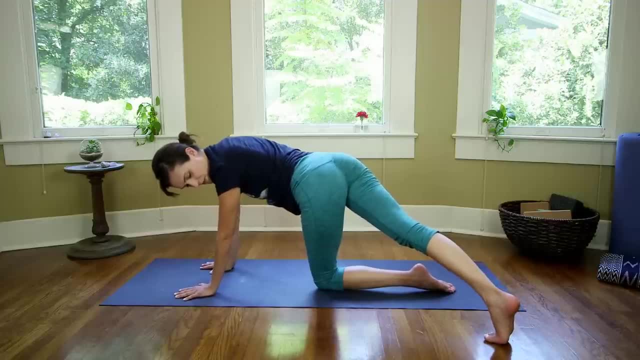 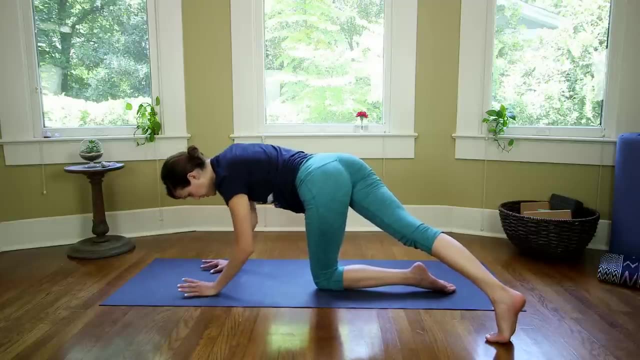 of your yoga mat and then take a look, Take a little gander at your right foot. If you were able to do the Dunda practice with us, this will help here. You can really see that line from the crown of the head to the. 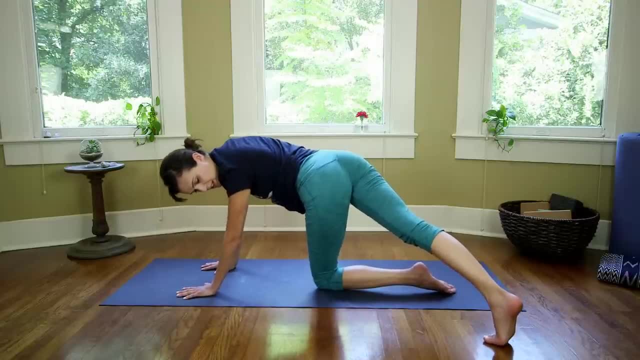 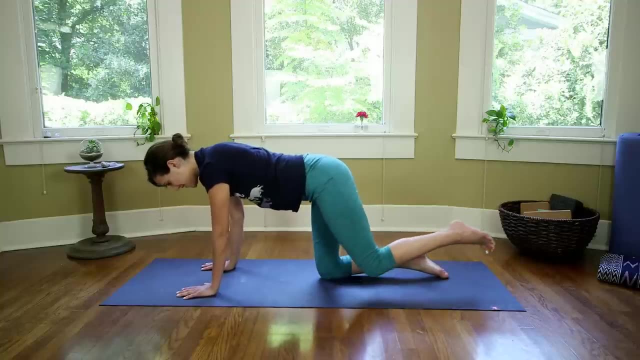 tip of the tailbone here. so we're not collapsing, We're really engaging. Stretch it out, stretch it out and then release back to center. and the same thing on the other side: We inhale, lift the left leg up, Square the hips and then take it over towards the right. 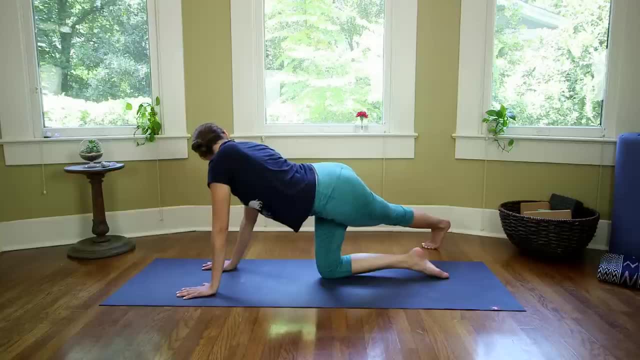 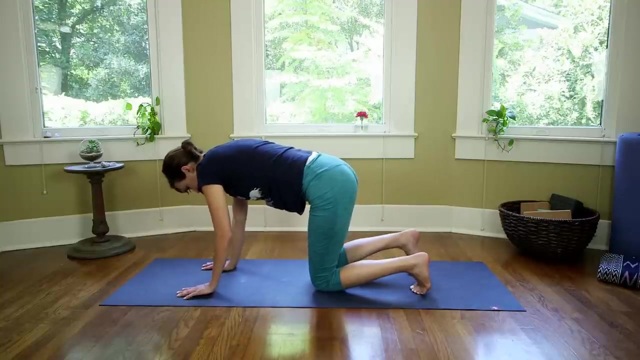 Take a look at your right- Excuse me, your left- leg. Press away from the earth with both palms, Stretch, stretch, stretch, And then we release Awesome. From here I'm going to curl the toes under, Take a deep breath in and then, nice and easy, keeping the knees. 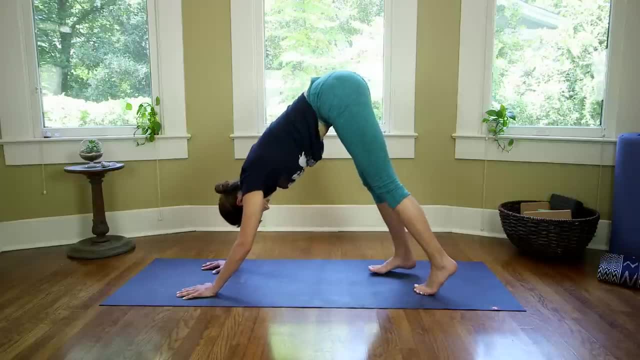 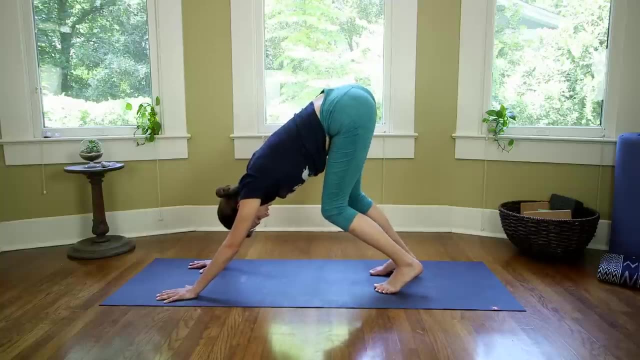 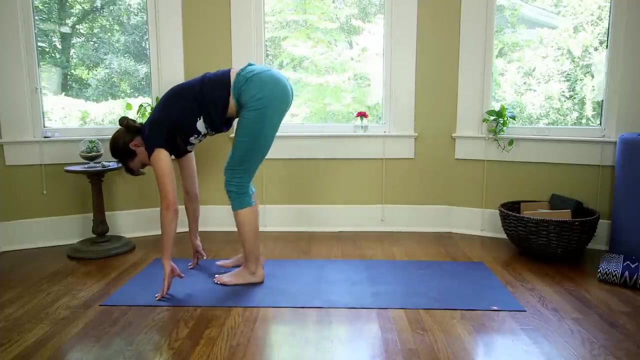 bent. I'm going to send it up to a downward dog, Pedal it out here, Soften the knees And then we're going to slowly walk it up all the way to the front edge of your mat, Take a nice forward fold and when you land, just you know notice. 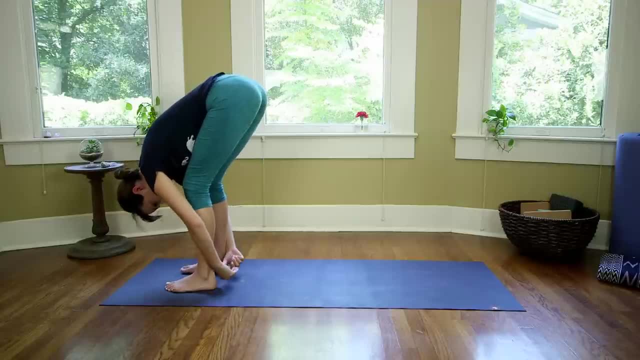 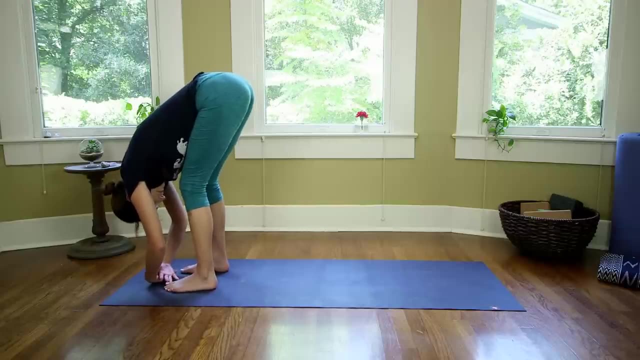 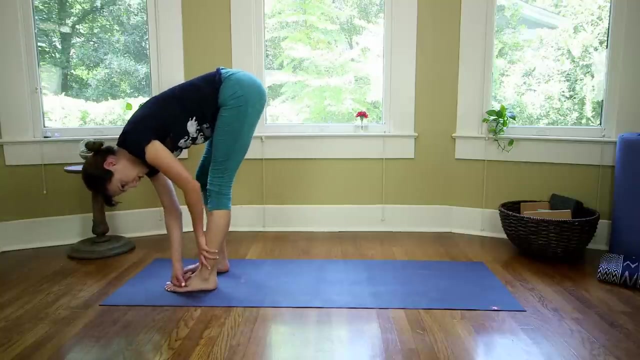 your breath, Notice how you might have stopped breathing and continue to breathe deeper and deeper as you let the weight of the head go. So we're really trying to awaken the breath and if that's tough for you, I just want you to know you're human. 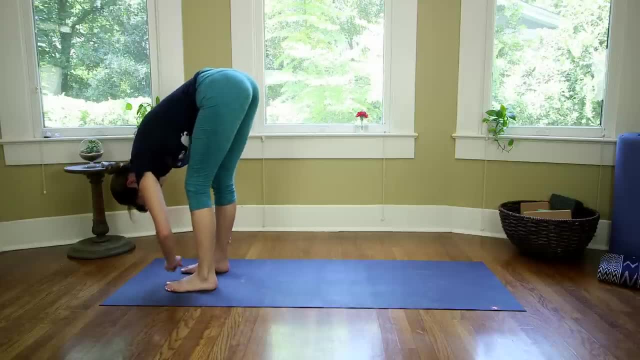 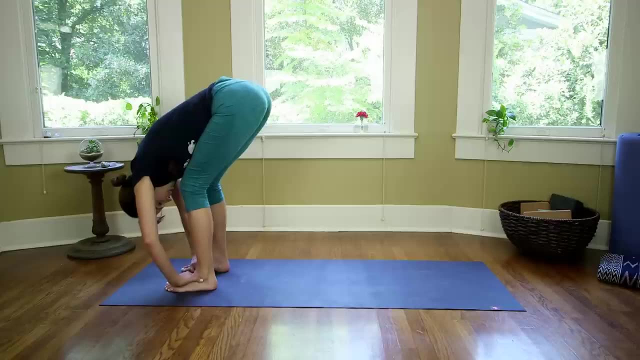 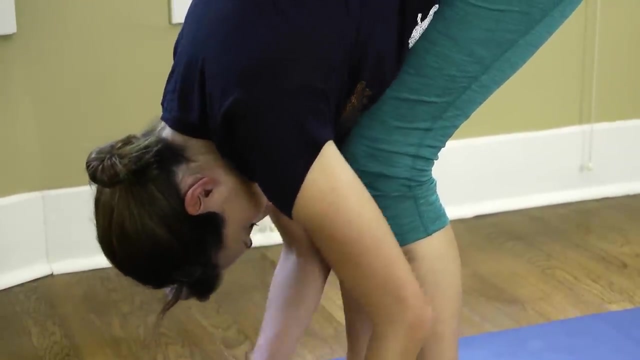 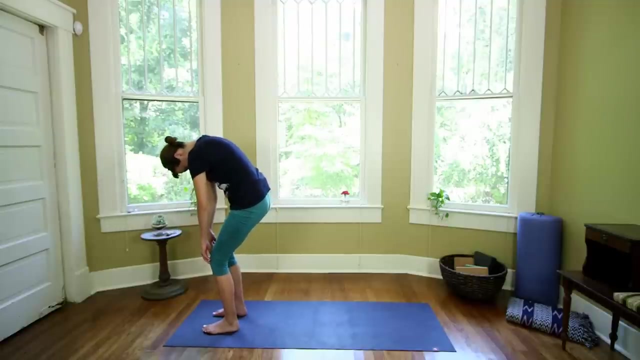 You're not alone. It's a super challenging thing to cultivate a more mindful breath practice. When you're ready, roll it up nice and slow. How slow can you go? Enjoy this. move all the way to Mountain. Keep the knees softly bent here as you roll up to a nice tall. 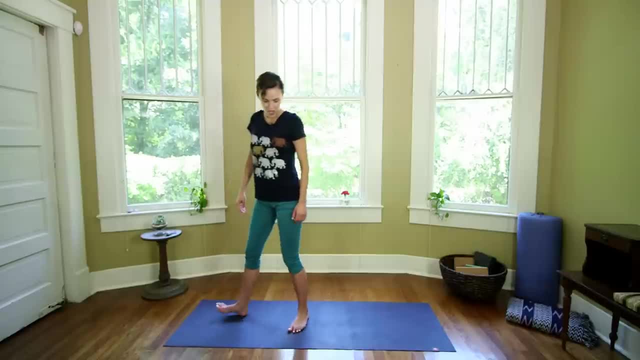 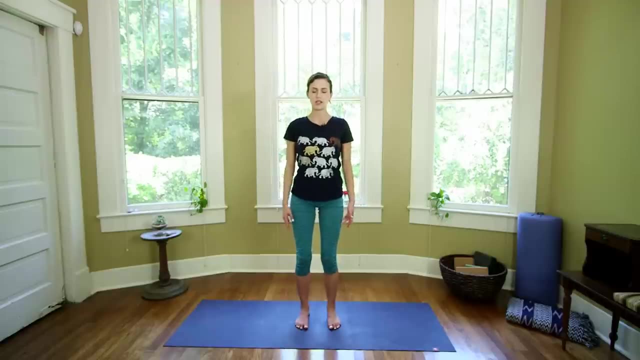 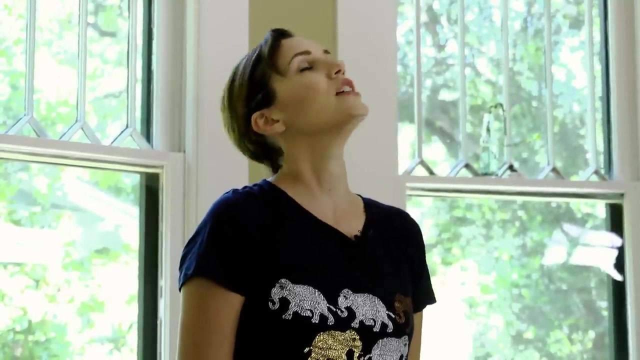 mountain pose, Lifting up through the crown of the head, and then going ahead and just kind of taking this opportunity to check in with your body today, whether it's looping the shoulders, drawing some circles with the nose, a little neck hygiene here. 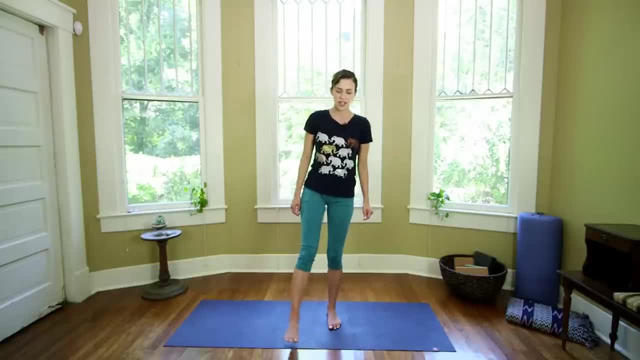 Maybe you know pressing into the feet, shaking out any leg cramps, rolling through the ankles a couple times the wrists. So go ahead and take a little freestyle moment to release that muscle. So really check in with your body and then we'll stand up nice and tall. 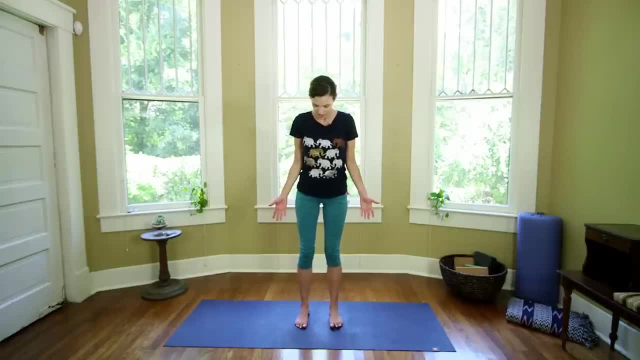 Toes pointing forward, feet hip width apart. So we're really stacking the bones here And then, when you're ready, just getting used to moving with the breath And just going back for a second. stacking the bones is so important because, you know, our habitual selves kind of want to take over. 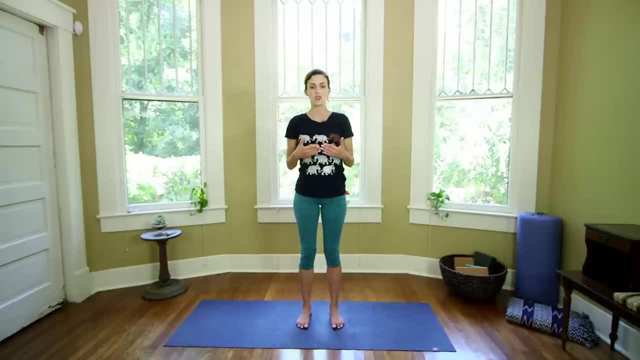 especially when things begin to move at a faster pace, as they do in vinyasa. So the more attention to detail we have now, while we're kind of going through the basics And really building the foundation of our practice, the better. So when you feel like you have a nice foundation, really pressing. 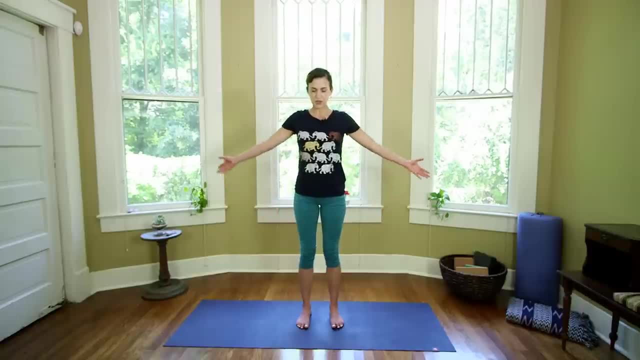 through all four corners of the feet. just go ahead and, nice and easy, reach the fingertips all the way up towards the sky and take a deep breath in, And that's it. Exhale, let it go And again full breath capacity. 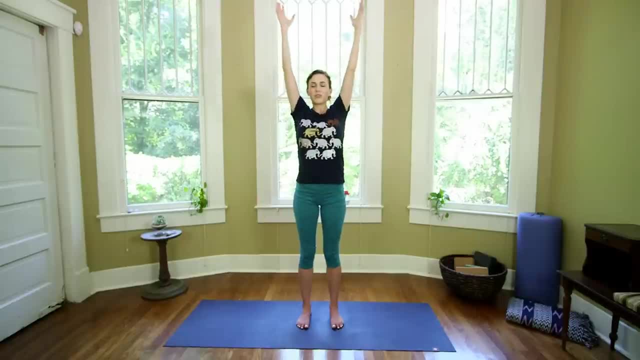 Inhale, reach up, Reach until you can't breathe in anymore And then exhale. let it go. Couple more. Try closing your eyes or just softening your gaze, Just going inward, focusing on the breath. Inhale: 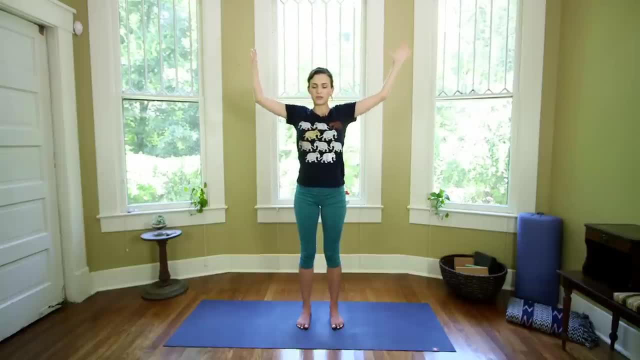 Exhale, get used to really moving with your breath, See if you can let the breath fuel the movement. And after you've kind of found that like synchronization- or at least tried- we're going to add one more thing to this So you can stay just kind of doing this flow here, synchronizing the 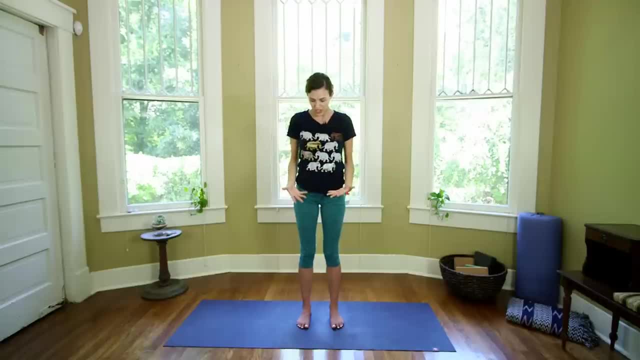 movement and the breath, the breath and the movement. Or you can begin to lift up on the toes, So we're practicing a little balance here too. Inhaling This also just requires us to kind of slow it down, so we have more. 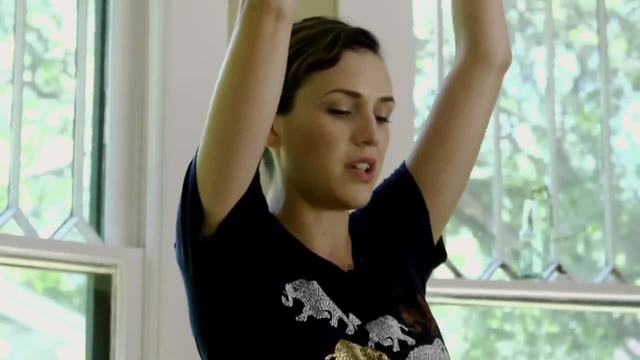 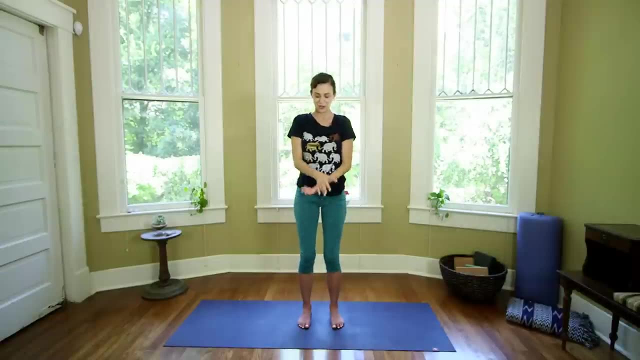 control over the breath and more control over the breathing. More breath and more control over the movement. Inhale, Exhale, slowly release. Let's do one more, spreading the fingertips. Exhale back down to Mountain. Draw the palms together at the heart. 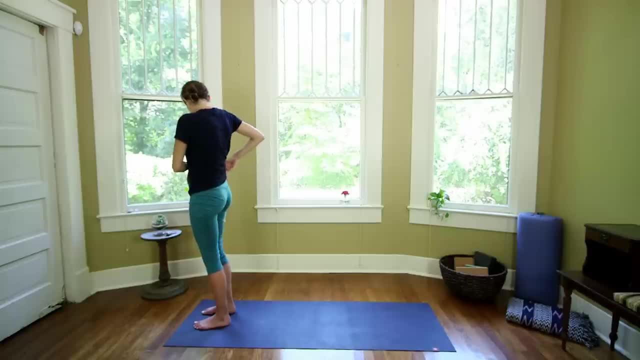 And let's keep playing with this Moving breath and movement together as one. Let's see what happens. Inhale: soft knees. Reach it all the way up, Moving nice and slow today. Exhale down: you go Forward, Fold. 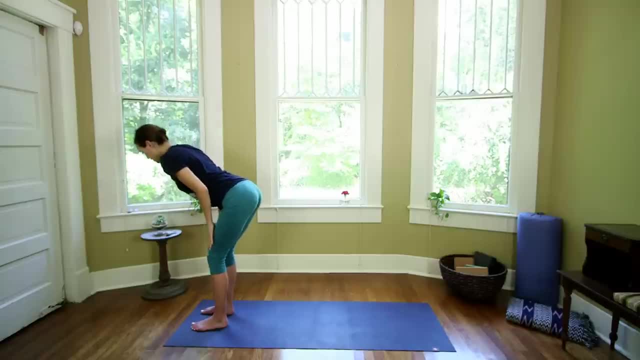 See if you can move with your breath And it's almost like we're moving through water today, Not because we want to be weird, but so that we can really just kind of stay in control of the movement and of the breath. Also, really great if you're a beginner, to just take it nice and slow. 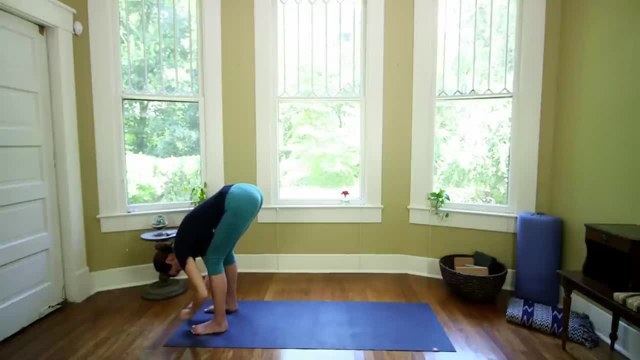 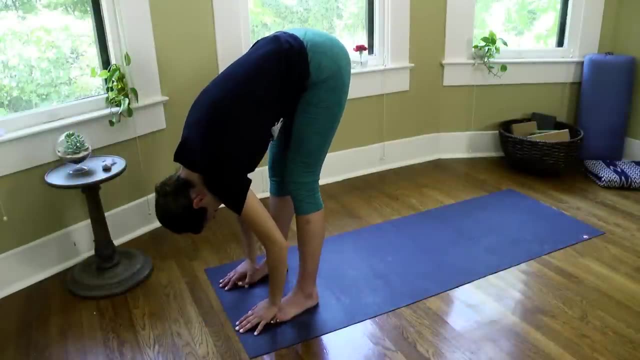 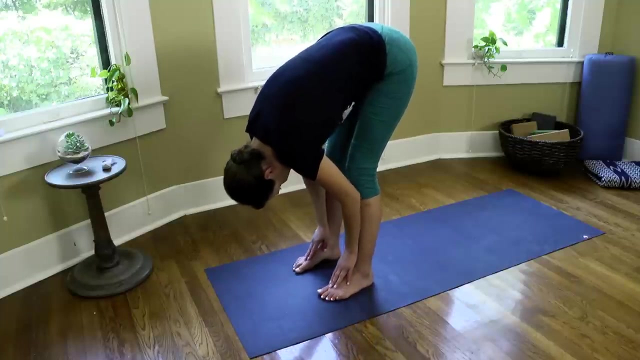 allowing the muscles that have been tight for so long to reawaken and stretch out. From here, I'm going to inhale and lift up to a flat back position. Now, what that looks like today is this: Sliding the palms all the way up the shins, all the way up the knees. 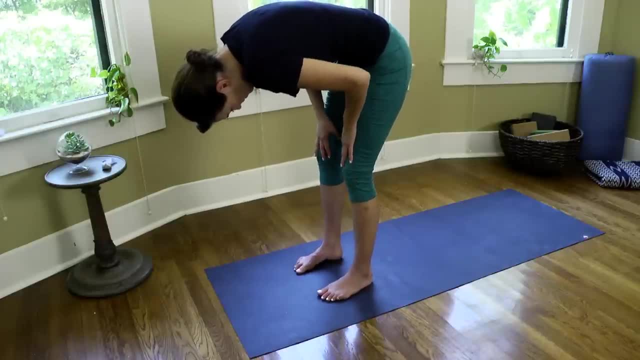 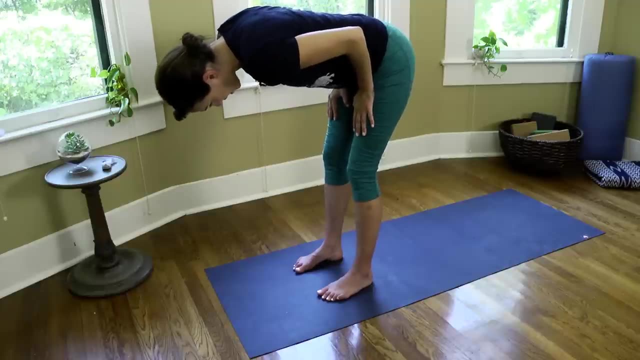 We kind of draw energy up through the legs as we do this. Just a little bonus tip. And then I'm going to loop the shoulders, pull the elbows back and find extension through the crown of the head, Kind of like I'm creating the number seven shape here. 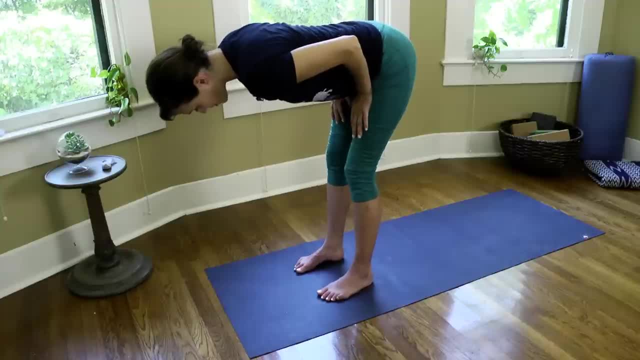 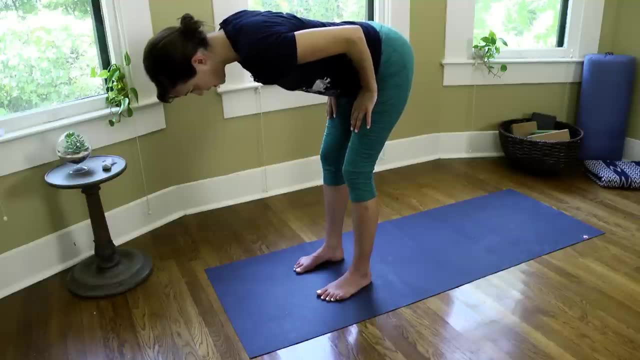 The legs might want to lock here, especially in certain body types. So just keep a soft bend in the knees, Everyone. draw your navel up towards your spine. This is hard work And we're going to draw the shoulders away from the ears. 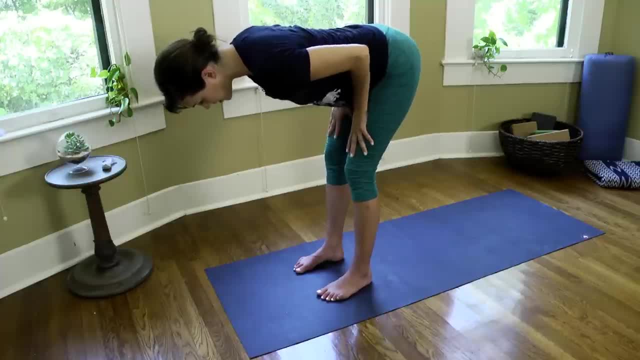 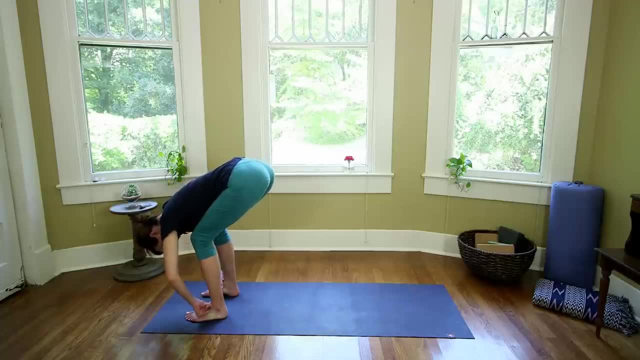 Take one more breath in here And then use your exhale to slide back down to that forward fold, Bend your knees super generously to give your lower back some extra special love here And then, if it feels good, you can grab the elbows. 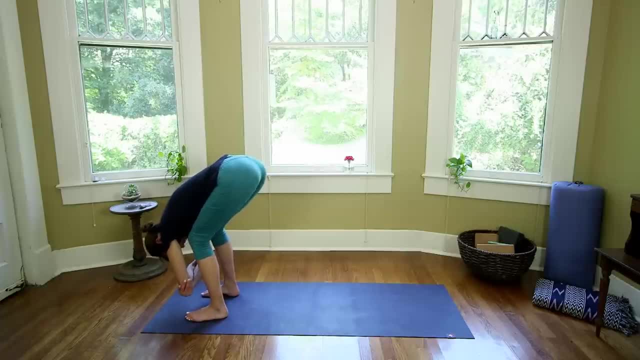 rock a little side to side, Keep breathing nice, long, smooth, active breaths best you can, And chances are- you know you will stop, And so we're just going to make it about coming back to the breath each time, even if you have to do it a million times. 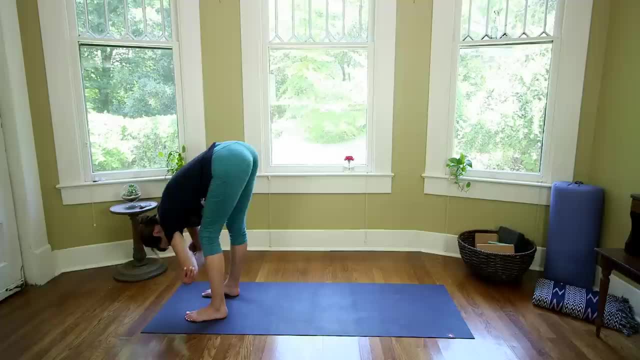 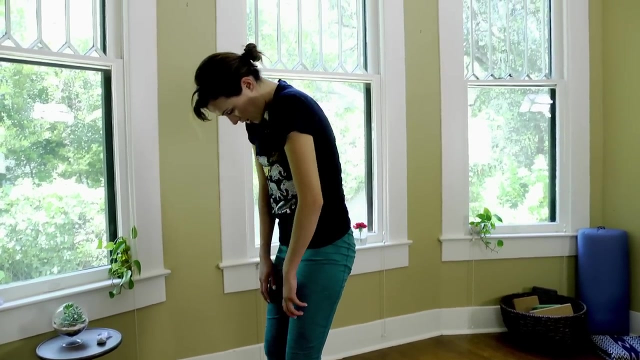 No worries, That's what the practice is all about. Then release the arms and slowly roll it back up once again, Press into all four corners of the feet And again we'll take a deep breath in and inhale, Reach up towards the sky. 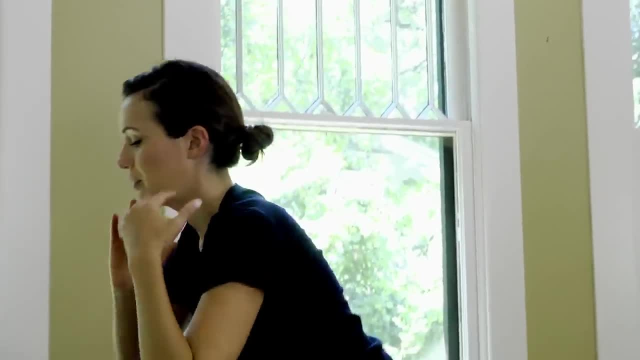 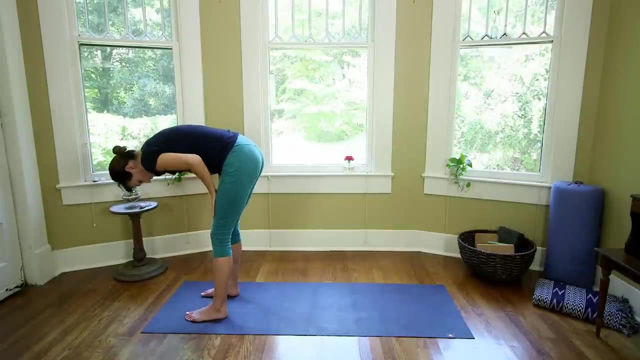 Exhale: Soften through the knees and down you go, Rain it down. Inhale Halfway, lift. Palms slide up to the tops of the thighs. We're just going to pause here and work on this shape, finding that length through the crown of the head. 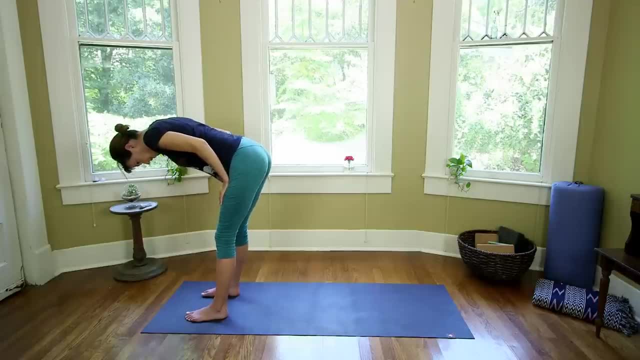 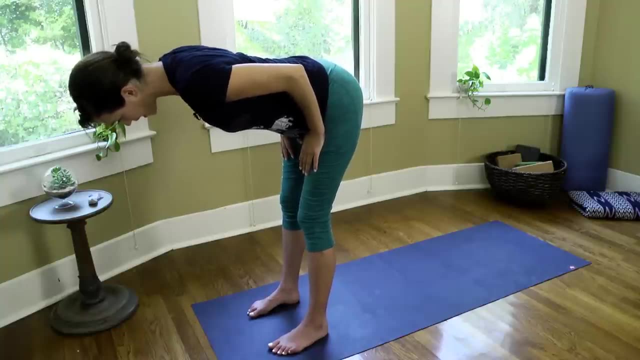 So usually the neck wants to kind of spill off like this. So remember that the neck is an extension of the spine. Remember not to lock your knees. Take a deep breath in, Pull your elbows back And then use your exhale to slide it down. 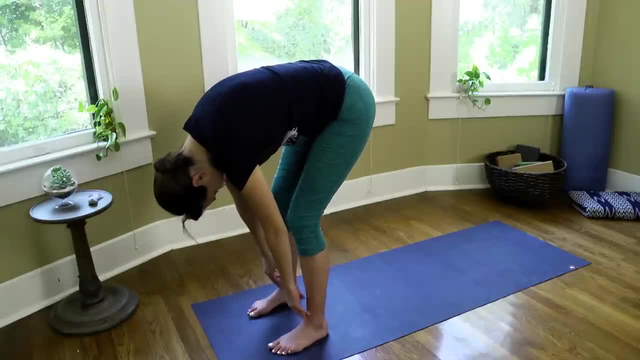 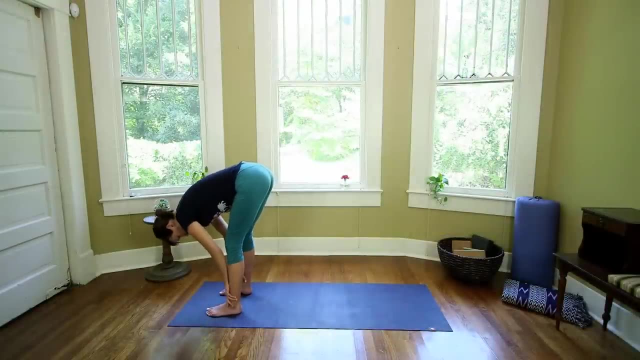 Great, Rolling up one more time, just like this Flat back position And then use your exhale to fold. Awesome. This time we're going to bring the fingertips to the mat, Walk the feet in just a hair And then, on a big breath in, send your right foot back. 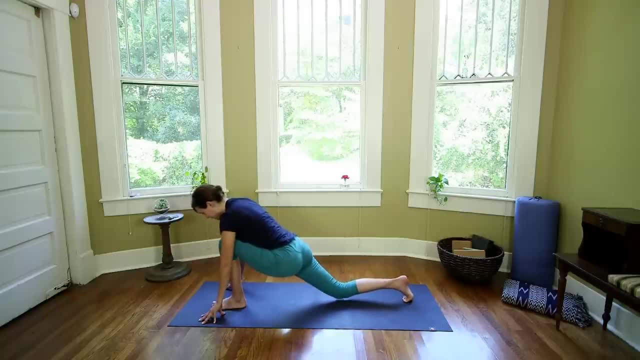 On an exhale: lower your right knee, Inhale, Open your heart, Awesome Exhale, Inhale, Exhale. Plant the palms And we're going to step the left knee back to meet the right. 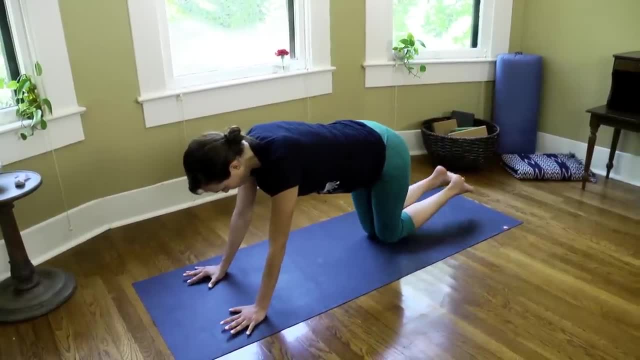 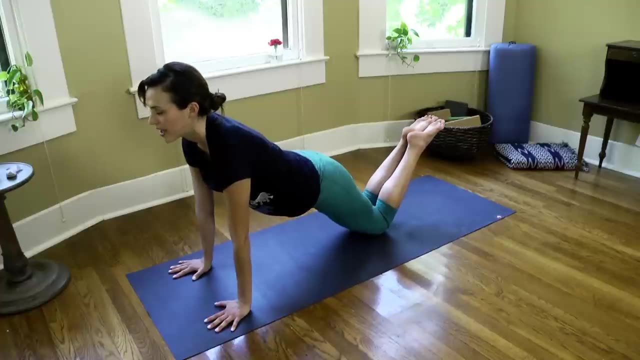 Cool, Catch your breath, Gather your bearings And we're going to come to kind of a half pushup here. Inhale, Open your heart forward. So really let the chest open. Exhale. Bend the elbows Slowly lower down. 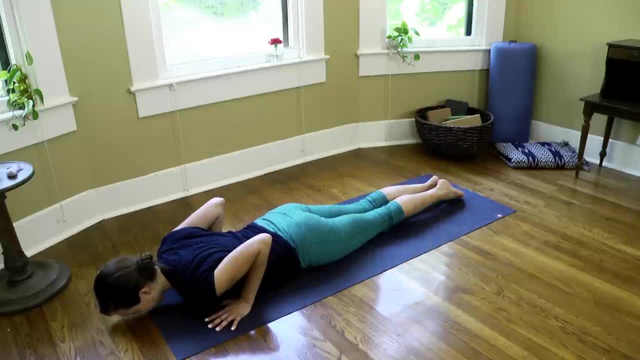 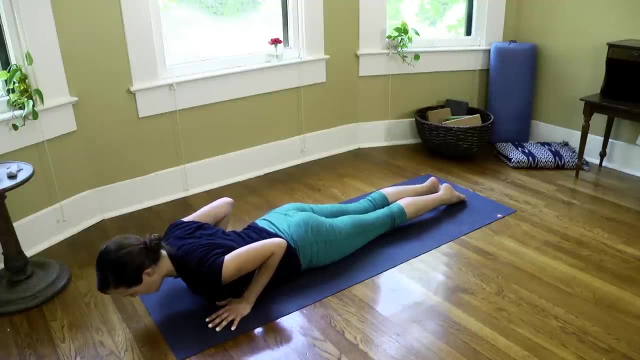 Stay down And inhale. Lift the heart up. Lower the legs, if you haven't already. Cobra, Exhale, down. Keep your cobras nice and small here. Inhale, Lift up, Especially if you're new to the practice. 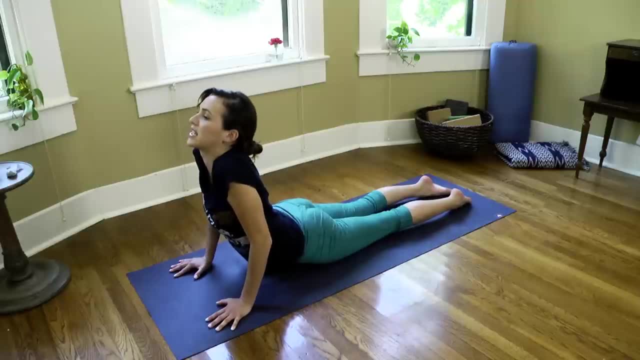 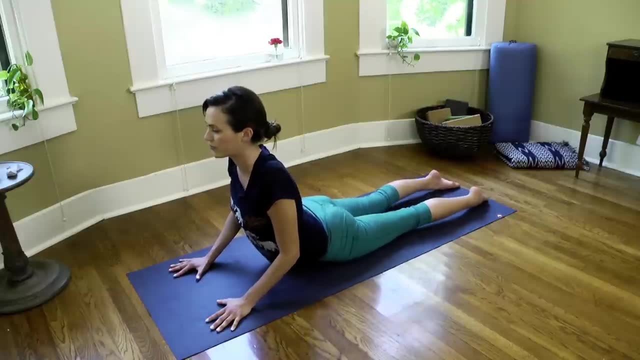 there's this tendency to kind of want to recreate the shapes that we see, And then this ends up happening because it takes a long time to kind of get everything integrated and working, happy to kind of get here. So don't worry, I'm not like trying to call you out or anything. 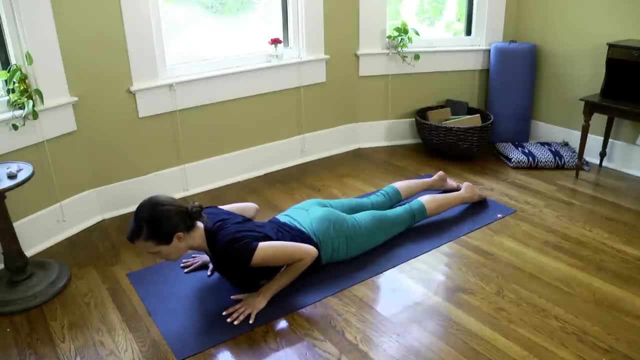 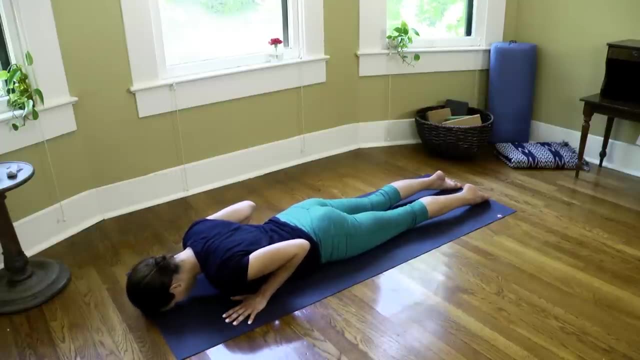 I'm just trying to help you. I don't want you to have any back pain or anything, So keep it nice and low: Inhale, Lift, Exhale Release. So we're doing this on our own here, really pressing through the foundation. 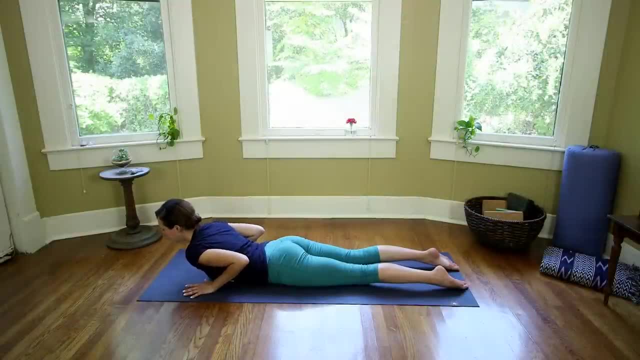 Inhale, Lifting up, Exhaling, Lowering down. Each time you lift up with the breath, pull the elbows back like little grasshopper legs, Press into your pubic bone and the tops of your feet So it's like a pump here. 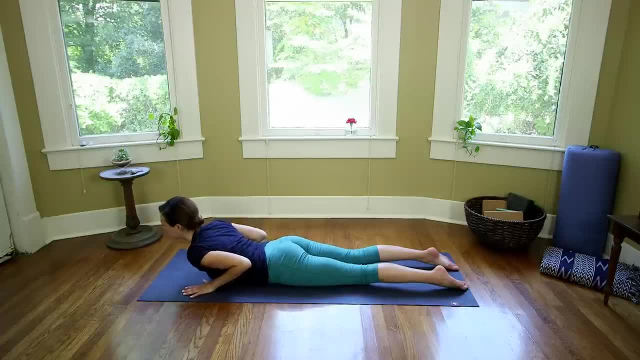 Inhale Lift And exhale Fall Curl. Let's do one more: Inhale Lift Baby cobra And exhale Release, Curl Cool. Curl the toes under, Lift the kneecaps. 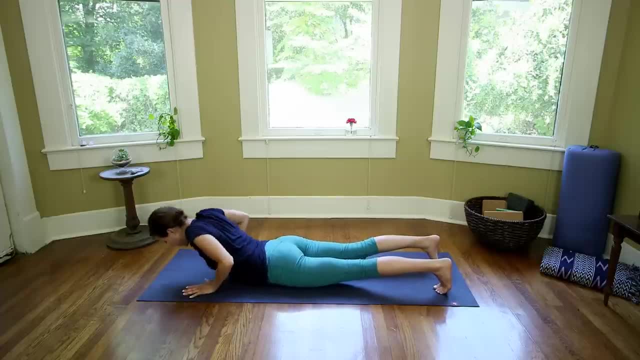 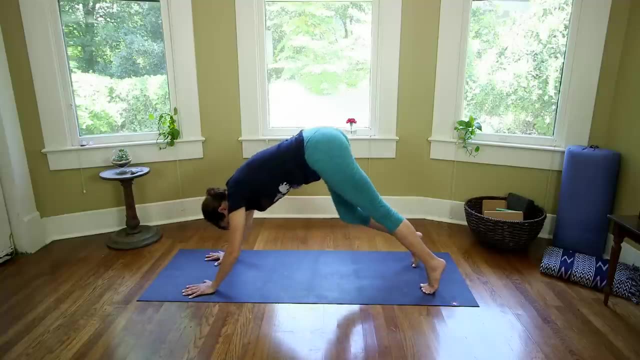 Inhale In Exhale. Press up to a pushup. You got it. It can always be at a half pushup. Inhale In Exhale to your downward dog Soften through the knees. 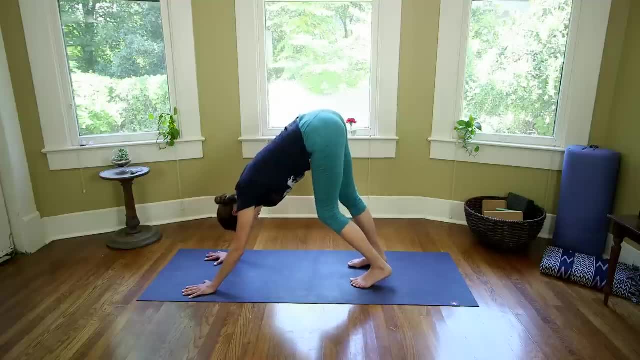 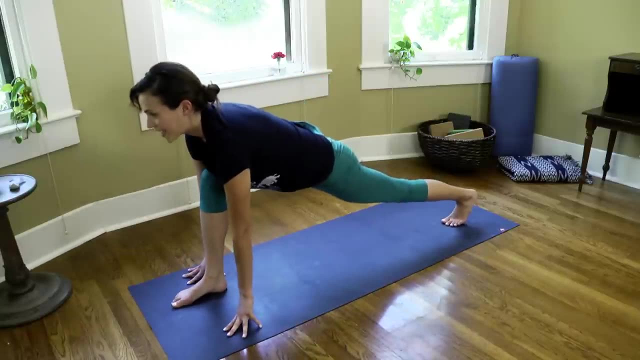 And then eventually begin to straighten it out. Awesome work everyone. Here we go On your next big breath in: lift your right leg up into your lunge, Exhale. Lower your left knee down, Inhale. Loop the shoulders. 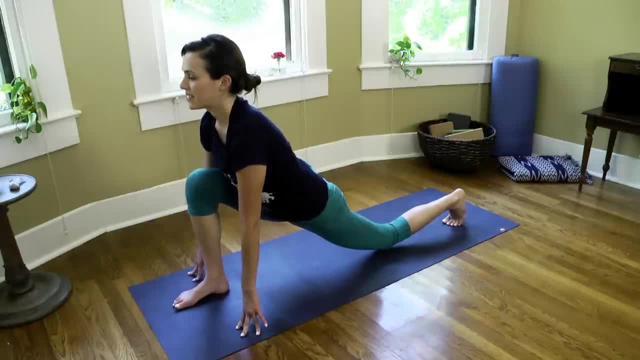 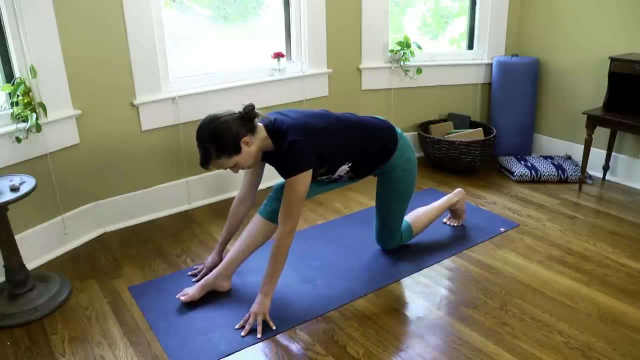 Open your heart, Take a deep breath in And exhale. Let it go Great. Inhale, Take your time. We're going to lift the back foot up to meet the front. Big breath in. And if that doesn't happen in one step, which it probably won't, who cares? 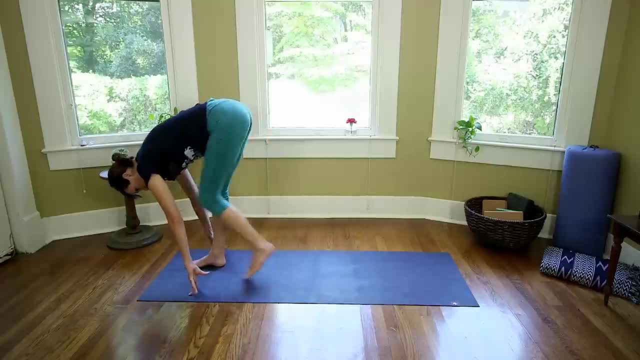 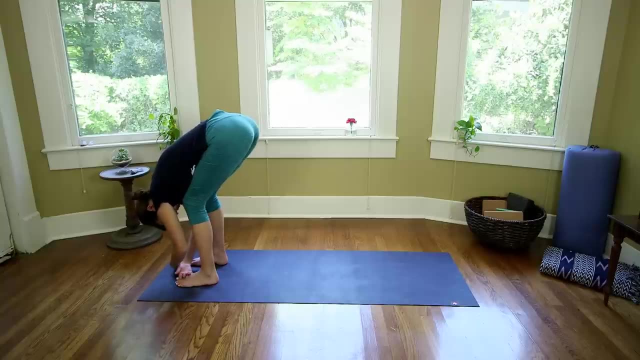 Take as many steps as you need And then everyone exhale forward. fold, Probably already there. so take a couple nice, long, smooth, deep breaths. Awesome. Inhale On your next breath, halfway lift. We know this position. 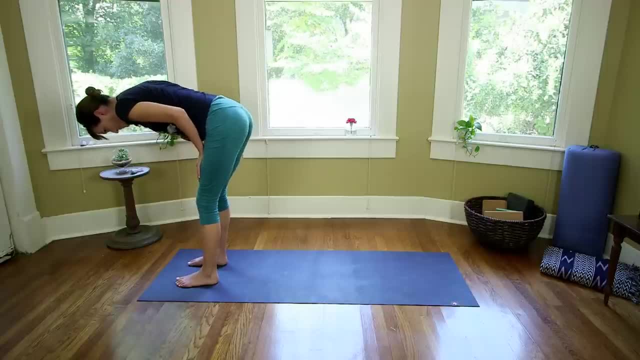 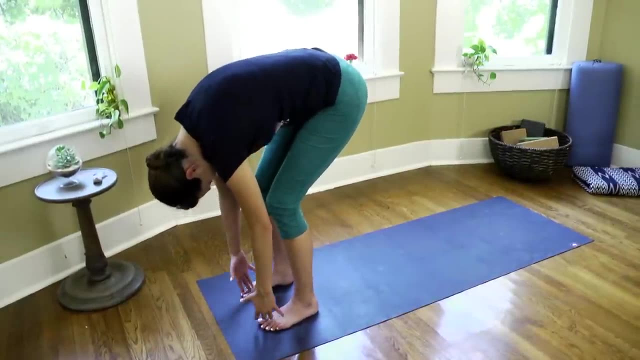 Just checking in, Staying curious, Experimenting And exhale Down you go. And then, softening through the knees, Pressing through all four corners of the feet, Spread out, Inhale, Exhale Down you go. 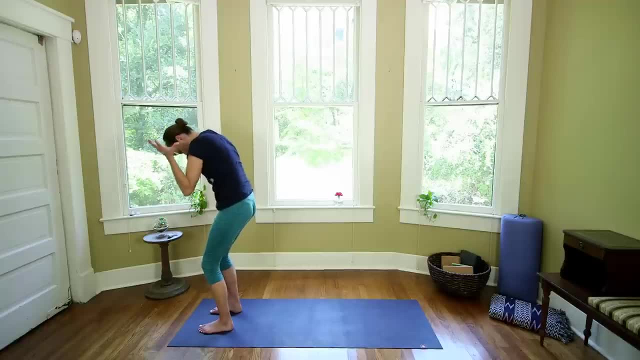 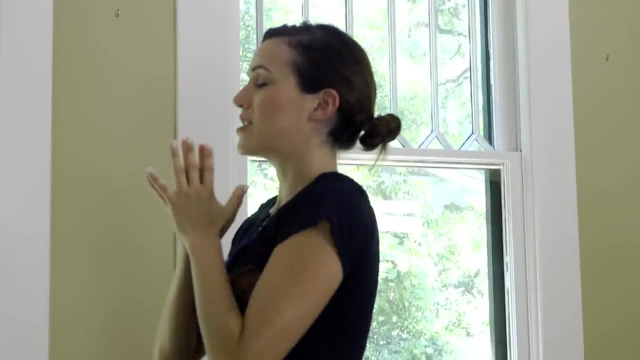 Pressing through all four corners of the feet. Spread your fingertips and begin to reach it up. Full body stretch. Should feel really good And exhale Hands to heart: Awesome. Just take a second to catch your breath or observe your breath. 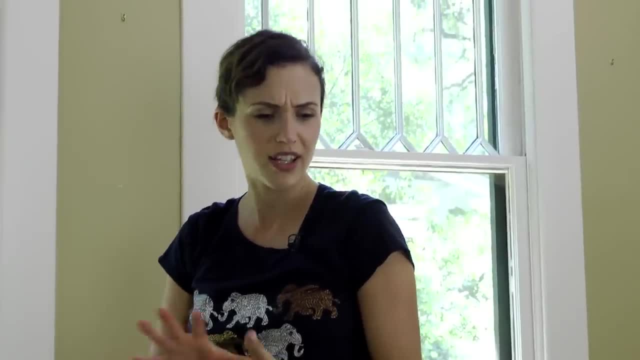 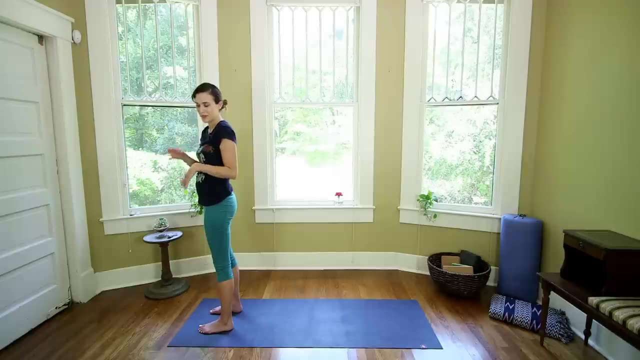 You know, getting used to moving with the breath in this way is actually like a really intricate thing. So we go to vinyasa class and we're like expected to just like perfectly sync up. So I think it's really nice to actually break it down like this. whether you're a beginner, 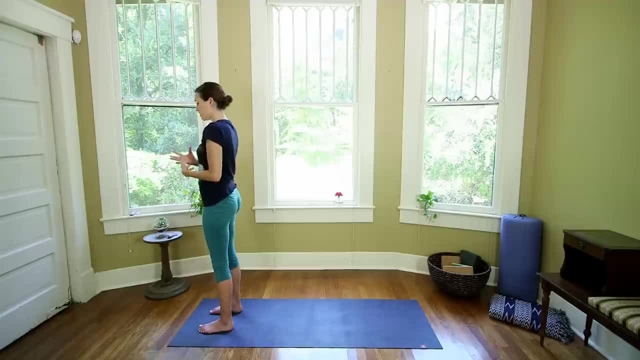 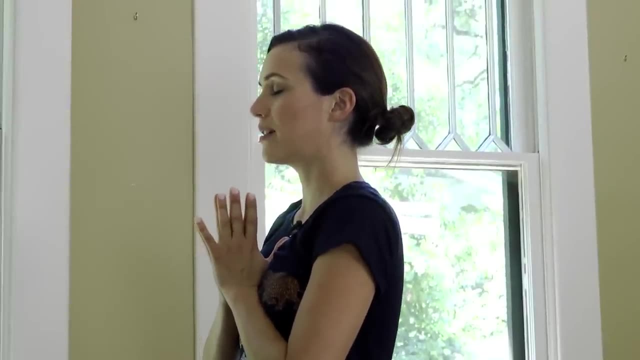 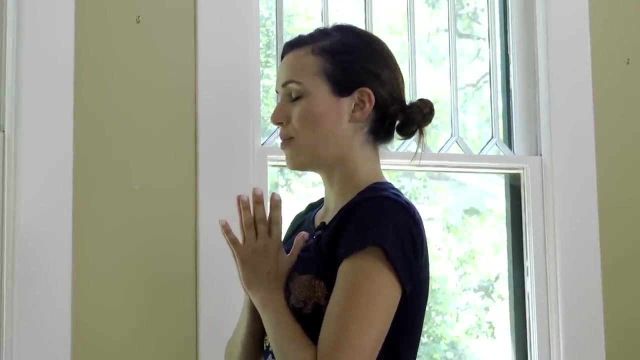 or not, just to kind of slow it down and remember: ah yes, synchronicity. So taking a second here to just observe the breath. If you're brand new to the practice, you need a sip of water right now. go get your sip. 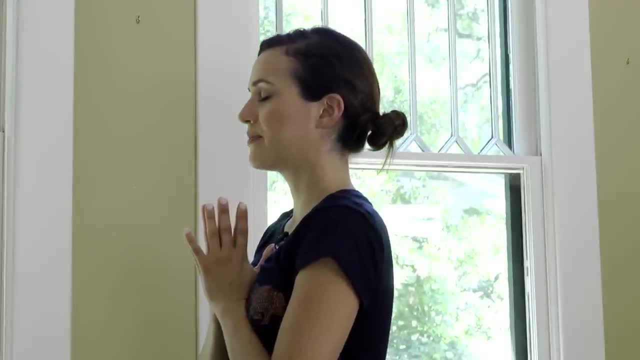 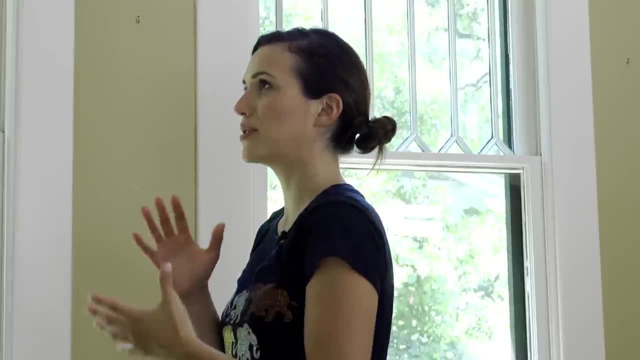 of water. I mean, it's really your home practice too, so you can kind of take what you need, That's when you return to the mat, Like when you're really listening to your body. A lot of yoga for beginners is just about like learning everything the right way and 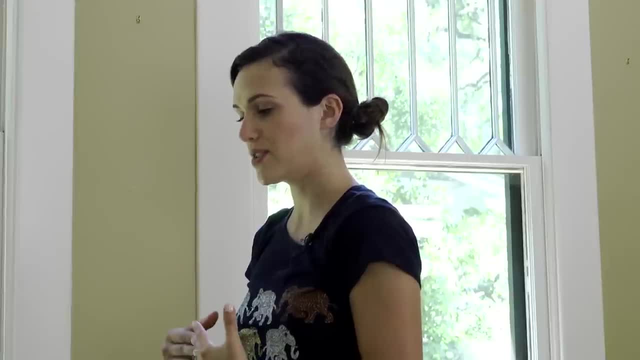 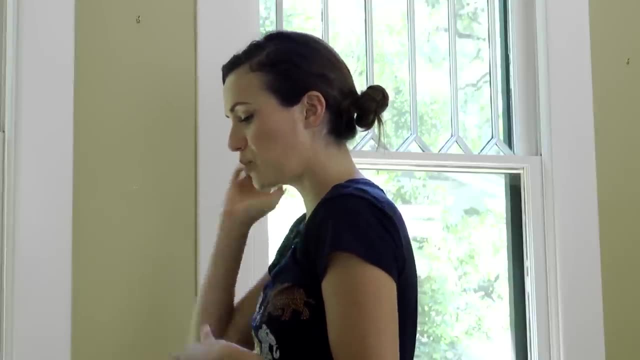 we forget to allow for permission to like make it so that you want to come back to your yoga mat, So okay, So we're just going to go through one more little flow here, Just practicing moving with the breath. So soft knees. 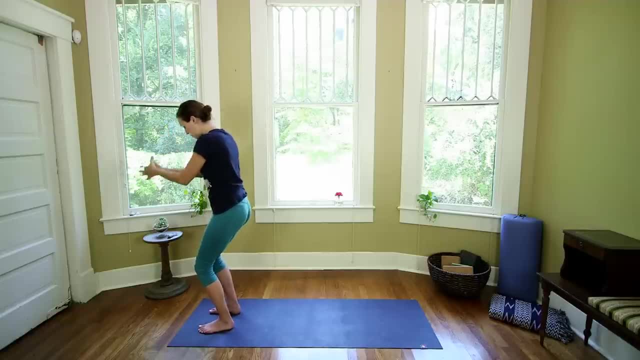 Marry the breath to the movement and the movement to the breath Best you can: Big inhale, Reach the arms up and overhead Full body stretch. Long exhale, Enjoy this move as you forward fold, Dive forward, Soft bend in the knees. 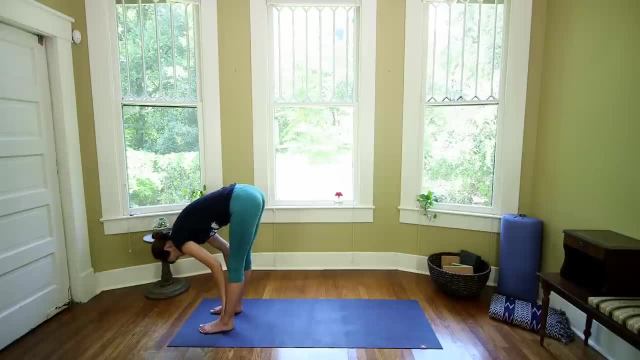 Take good care. Inhale Halfway lift. This time you might experiment with bringing the palms to the shins- Just another option instead of the thighs. Take a deep breath in here: Lengthen, lengthen, lengthen and then use your exhale to bow forward. 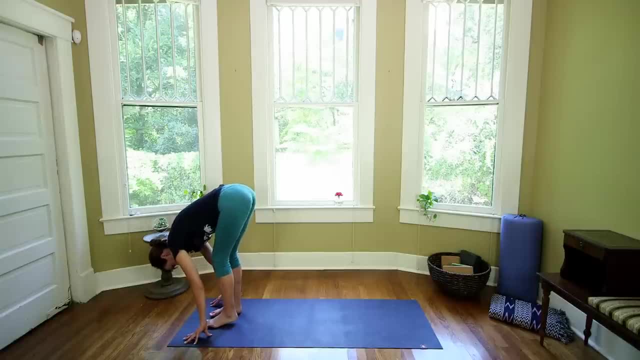 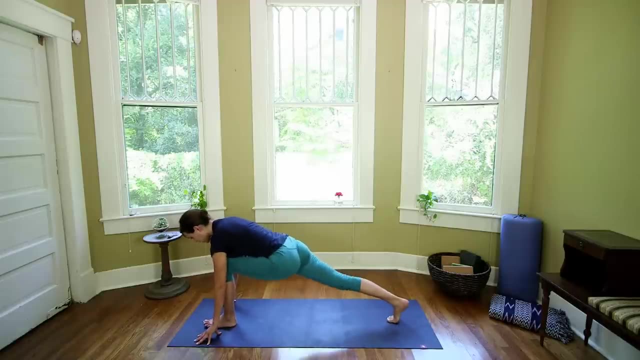 Again moving nice and slow. Walk the feet in just a hair Inhale. Step the right foot back into your lunge. This time you can keep the back knee lifted or you can lower it. Go ahead and let all the air out. 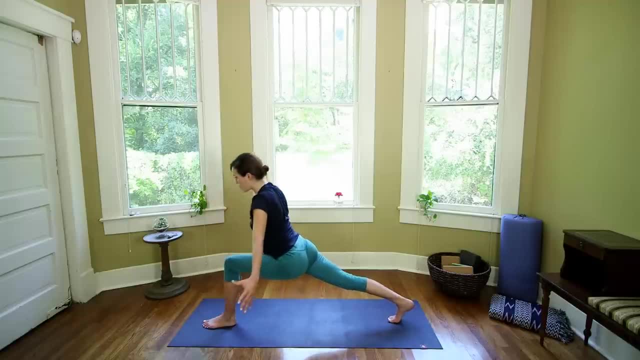 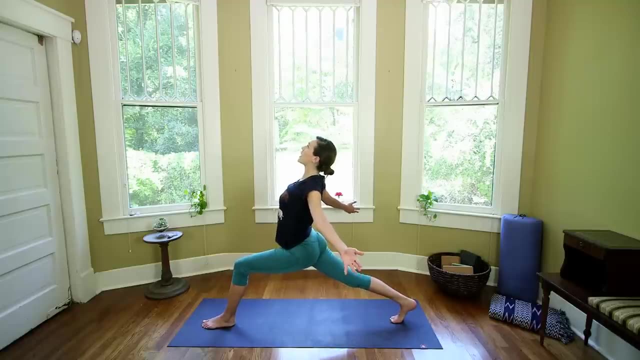 On your next inhale. open up the palms wide, Lift your heart, Press into your feet strong Again. we can also be on the knee here. Take a deep breath in Full capacity of breath here, as you open and expand and then exhale. 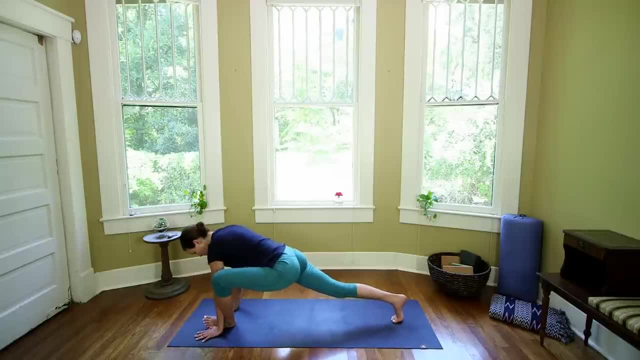 Back down. you go, Plant the palms, Walk the left toes or slide the left toes, excuse me, back to meet the right. Stay here or lower the knees like we did before. Inhale, Extend, Exhale, Slowly, lower down. 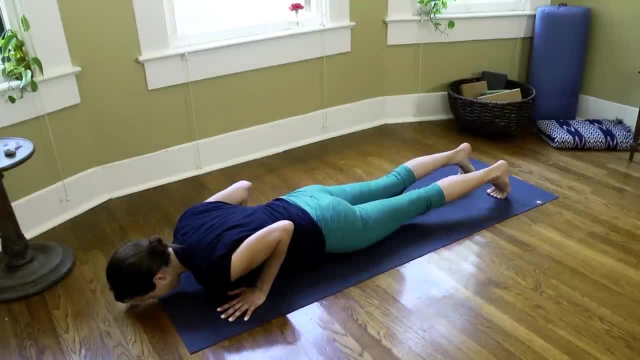 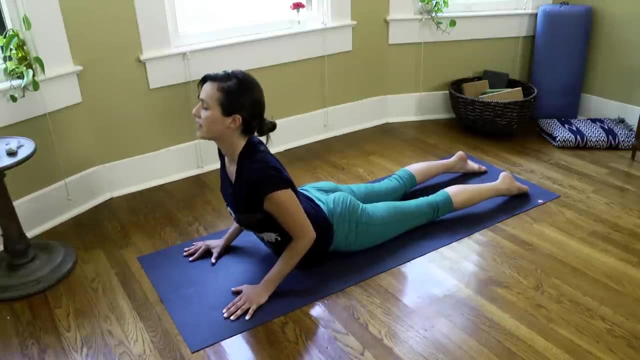 So we're doing it on the knees or we're lowering all the way down. Everyone hug your elbows into your side body and, on your inhale, lift up cobra, Move with your breath, Exhale, release, Inhale. curl the toes under. 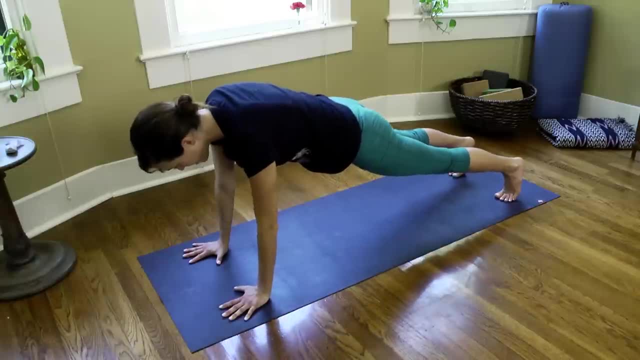 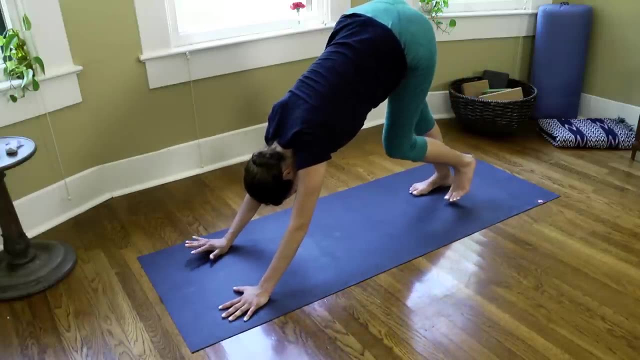 Exhale. Draw your navel up to your spine. Lift your kneecaps. Come up to push up plank. Inhale in Exhale, Downward facing dog. Awesome Inhale. Step your right foot up into your lunge. 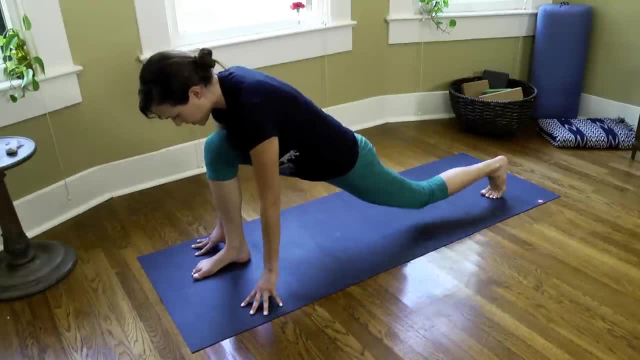 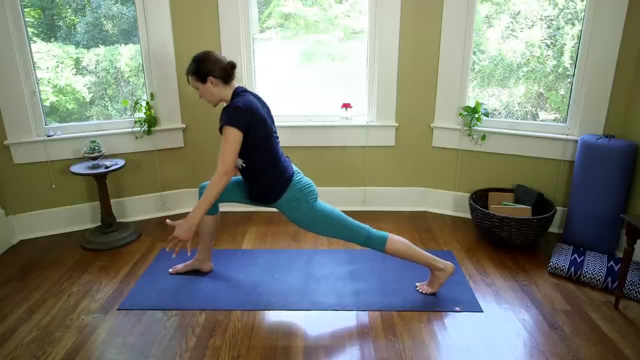 Again. you can lower the back knee here, Exhale, Or you can keep it lifted On your next breath in wherever you are. move at your own pace. We'll inhale, Open the heart, Expand Power up through the legs. 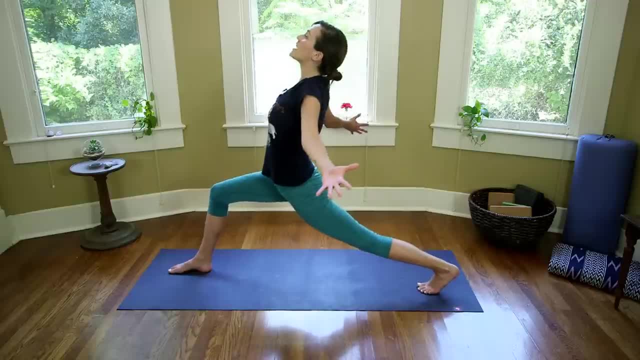 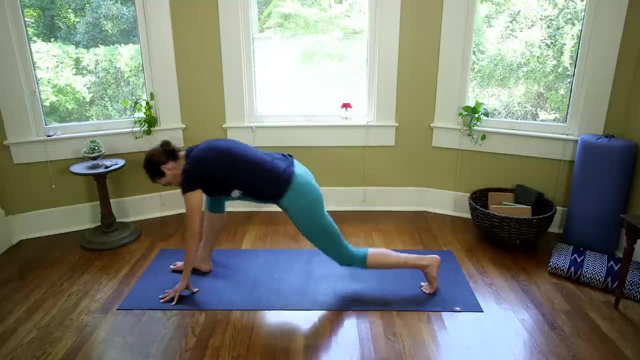 Open, open, open. Breathe in And on your exhale. let that be your cue to make your way back down. Awesome, Step the back foot up to meet the front. Take a big breath in Exhale. 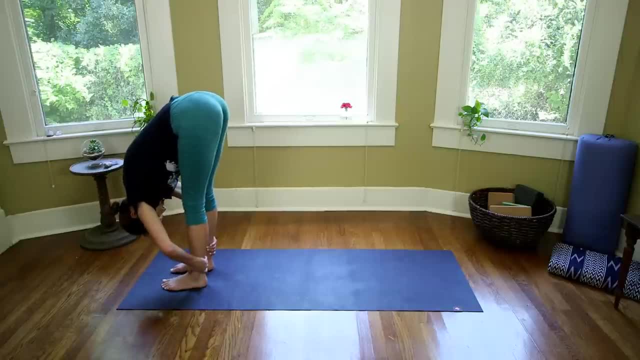 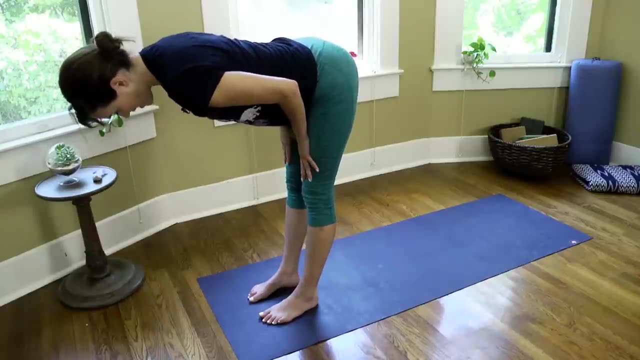 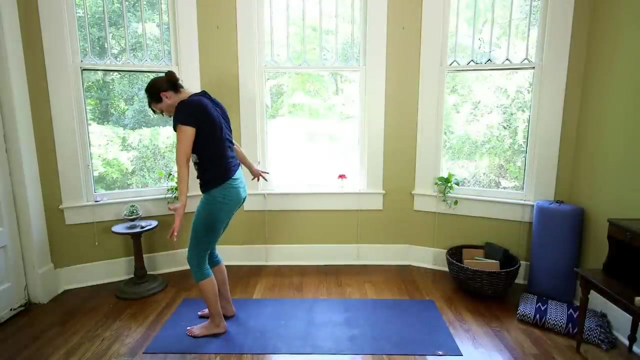 Down, Exhale Forward, fold- Awesome work. everyone Inhale Halfway. lift Palms on the shins or thighs. Exhale, Diving forward And inhale- Awesome work. everyone. Take the deepest breath you've taken all day as you reach your fingertips up towards the.